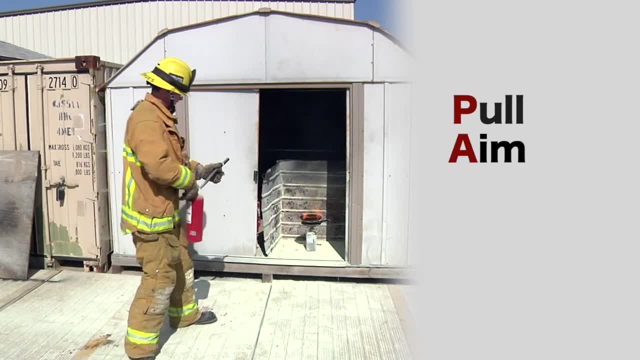 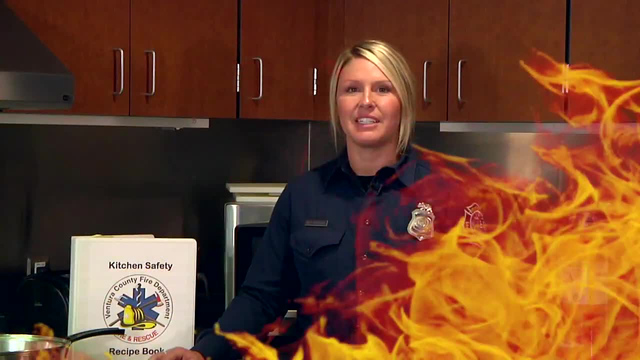 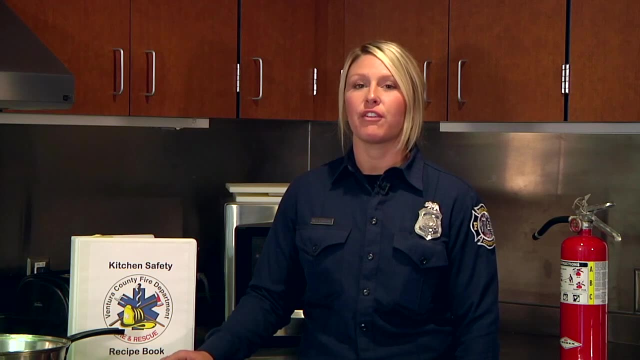 You're going to go ahead and pull, aim, squeeze and sweep, And that's how you put the fire out. Thanks, Mike. Now that we've prepared the kitchen for cooking, we're going to go over the five ingredients for kitchen safety. 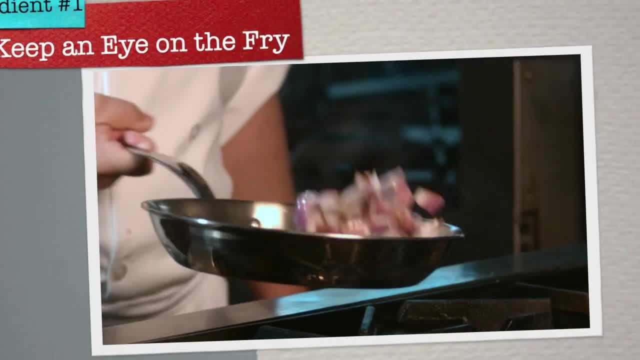 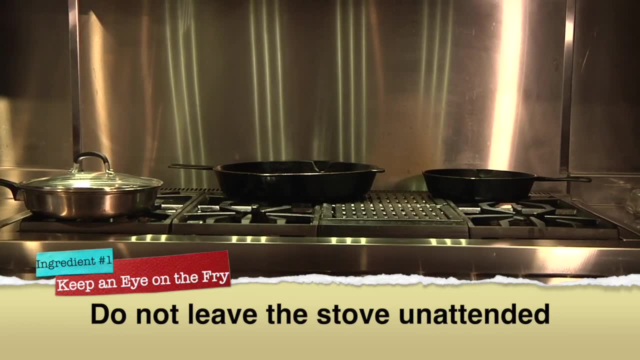 The first ingredient is keep an eye on what you fry. Nearly two-thirds of all kitchen fires start on the range or cooktop. Don't leave food unattended on the burners or the stovetop, especially if you are frying food. 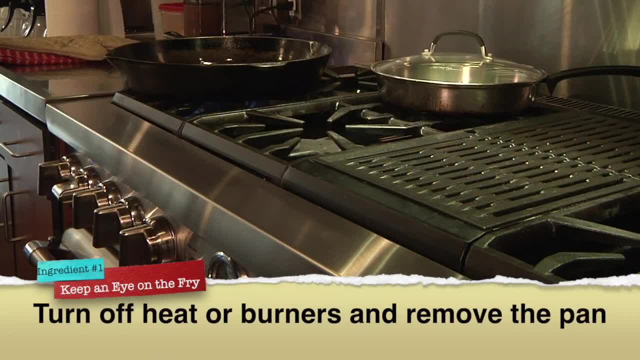 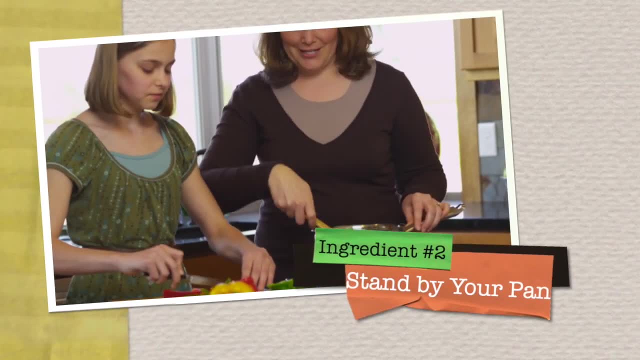 If you have to step away from the stove or leave the kitchen, turn off the heat or flame and remove the pan from the burner. The second ingredient: stand by your pan While cooking on the stove. use a pot holder or oven mitt to hold the pot handle while. 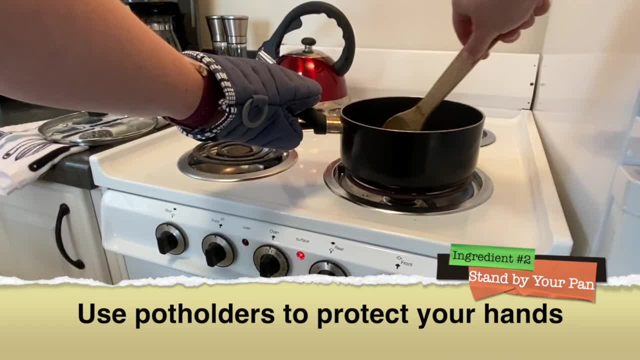 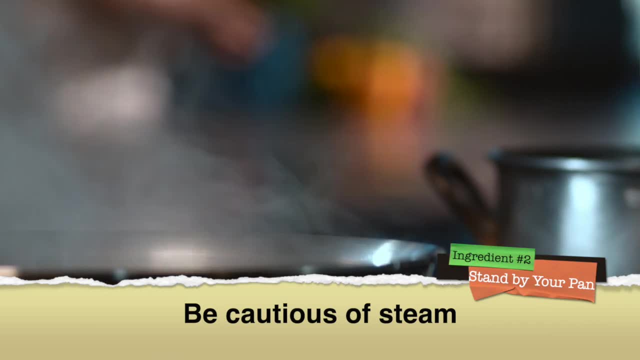 stirring the pot. to prevent burns. Do not stand with your face over a pot. when you are taking the pot, cover off The steam that accumulates can blow up in your face and result in burns. The third ingredient: turn pot handles towards the back of the stove. 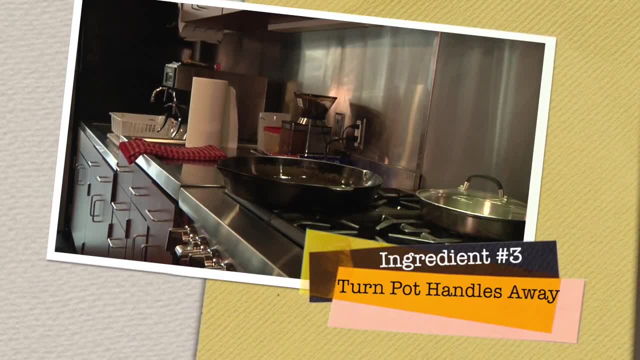 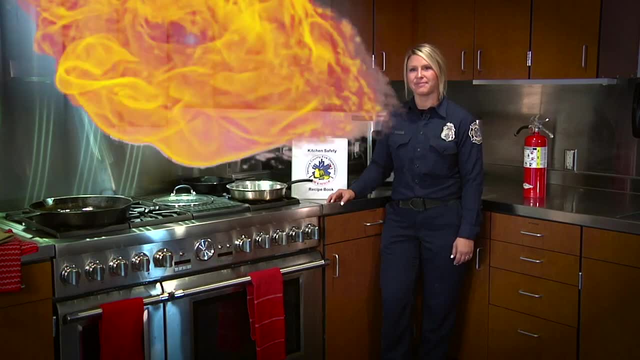 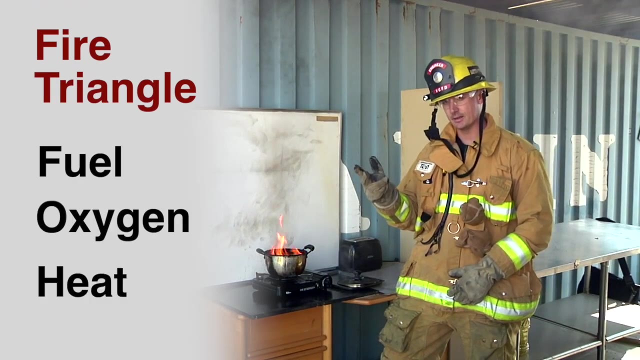 Turning the handles backwards helps prevent accidentally tipping the pot over. The fourth ingredient is to keep a lid or cookie sheet nearby. We're going to go back to engineer Mike to find out why Fire needs three things to exist. It needs fuel, oxygen and heat. 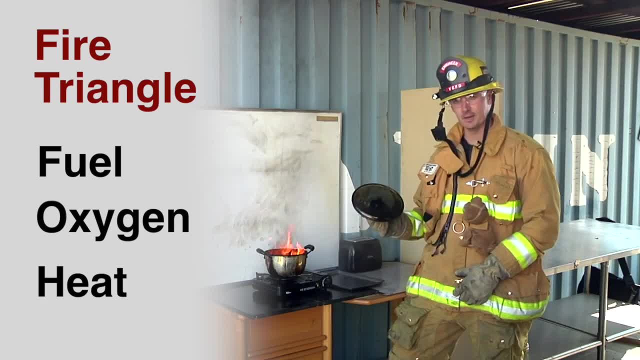 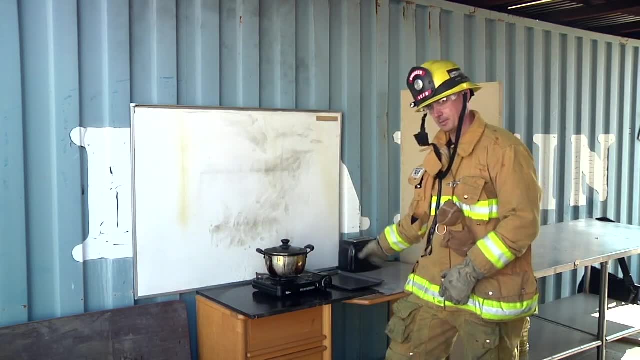 Here we have all three. I'm going to show you the simplest and most effective way to extinguish a grease or an oil fire, And that's simply to cover it up. You can use the lid from a pan, as long as it fits correctly, or a cookie sheet. 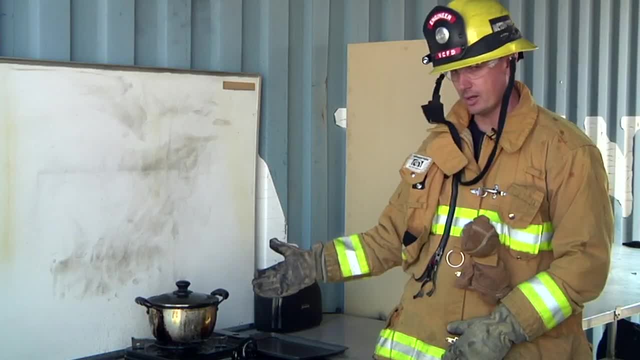 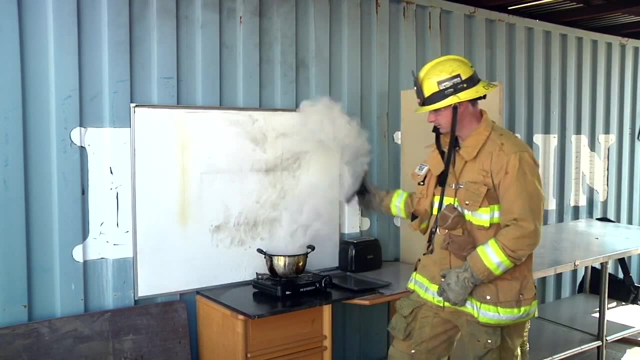 You're going to want to leave the lid on until it cools down, And always remember to turn the heat off also to the fuel. If you take the lid off too soon, it'll reignite, And that's how you extinguish an oil fire. 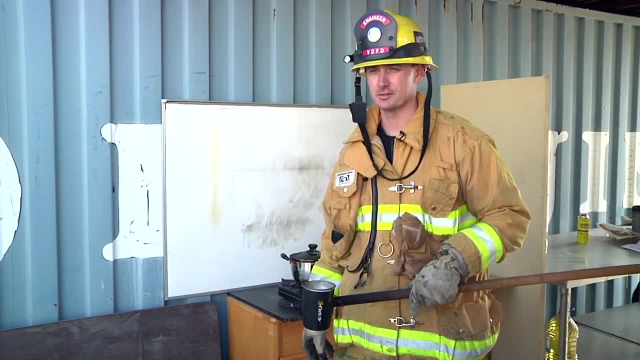 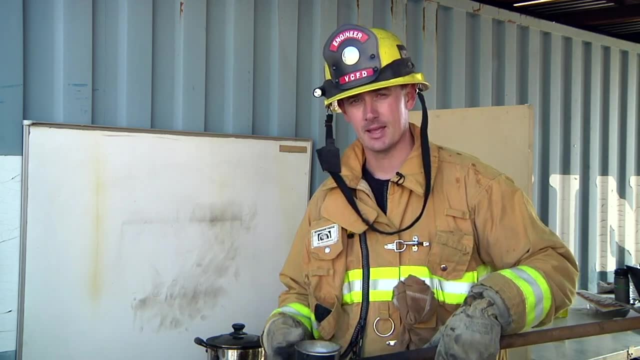 Adding water to a grease fire is very dangerous. The water is heavier than the oil, so the oil rises to the top, It doesn't mix with the oil and it converts the steam, carrying all the oil and grease which are now on fire out of your cooking utensil.